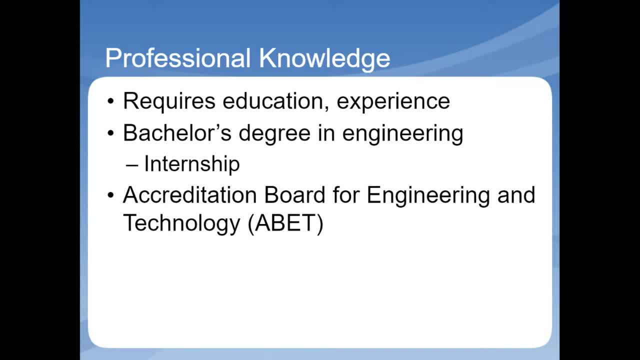 An associate's or bachelor's degree is usually required to become an engineering, technologist or technician. Most degree programs are structured with the same first two years focused on math, science and general studies and the last two years focused on specific engineering disciplines. 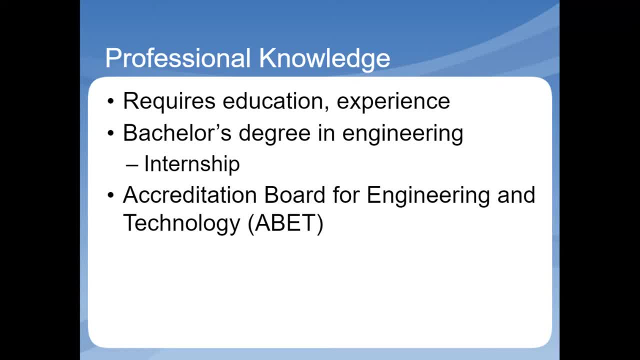 Many engineering programs also offer internships to give the necessary experience to be hired after college. Many programs are accredited by the Accreditation Board for Engineering and Technology, which requires students to graduate with a range of skills from applying knowledge of math, science and engineering. 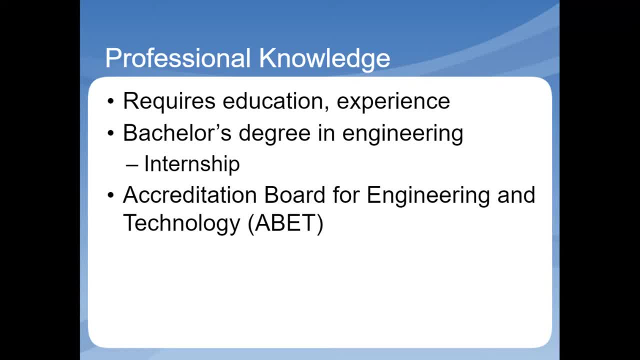 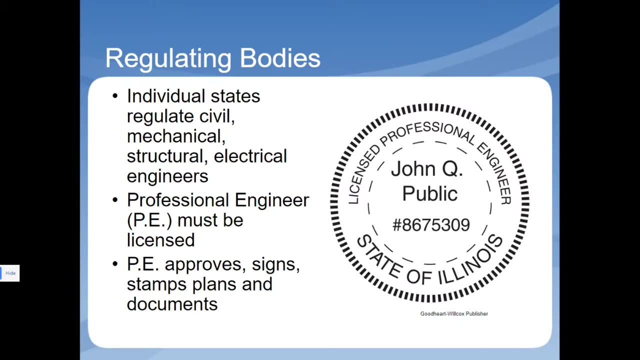 to conducting experience, experiments, designing systems and solving engineering problems. The work of many types of engineers is regulated by individual states. This is especially true of civil, mechanical, structural and electrical engineers. The title of professional engineer PE. 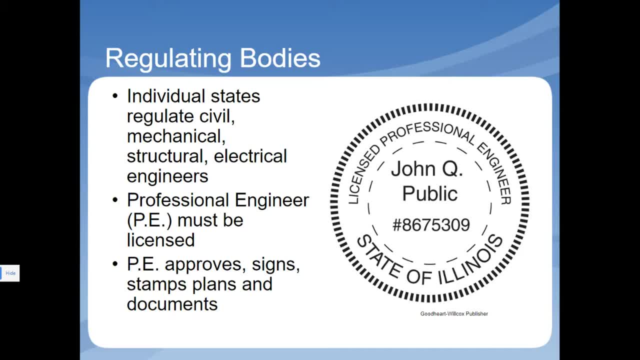 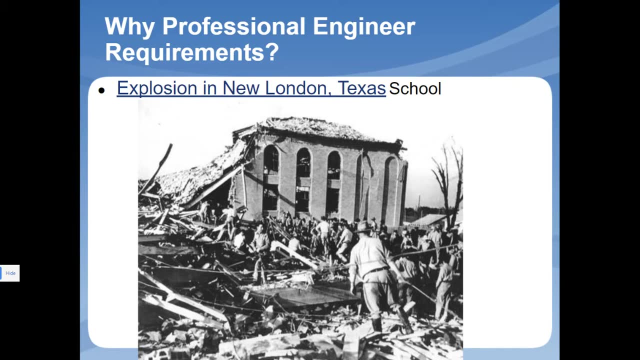 is an important designation because professional engineers are allowed to approve, sign stamp plans and documents. So why professional engineer requirements? Well, it all started with an explosion in New London Texas in the New London Texas school. The school opened in August 1936,. 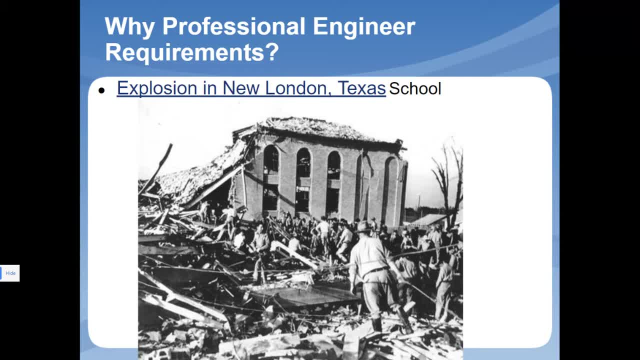 and during the design phase, school officials instructed the construction crews to tap into an oil field gas line to get gas for free, as it was estimated that the cost to heat the school would be in excess of $3,000 per year. The oil field gas was more unstable than commercial gas. 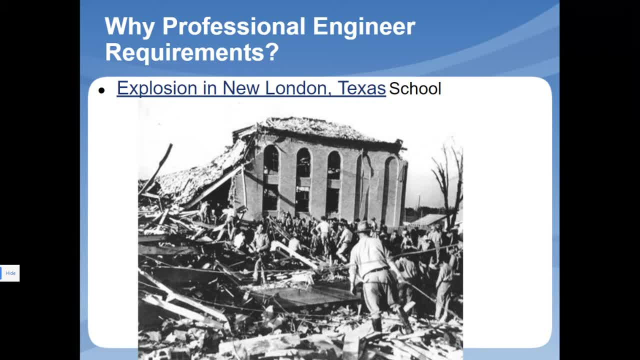 From January through March, teachers had tampered with the burners to adjust and regulate temperatures, which caused stress leaks on pipe connectors. March 18th of 1937, an instructor turned on a sanding machine in the shop, which was an area filled with a mixture of gas and air, due to a leaking gas pipe. 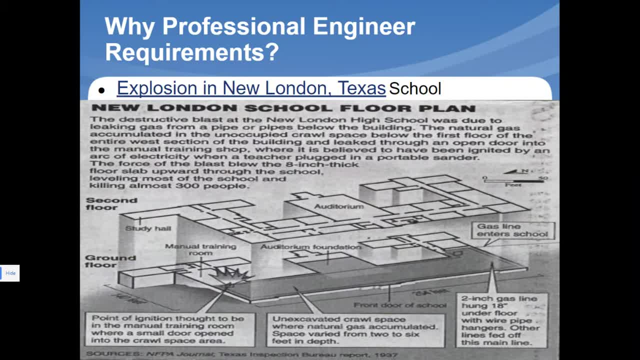 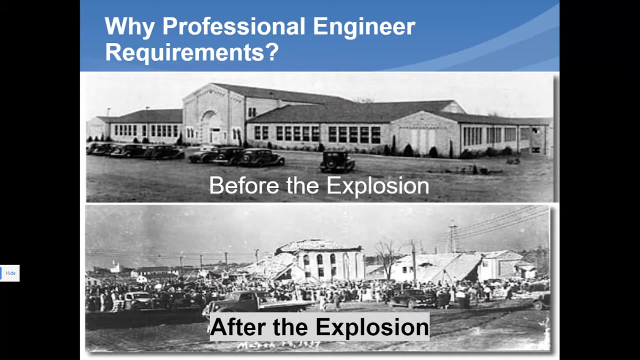 The switch ignited the fumes and carried the flames to a space beneath the building which was 253 feet long and 56 feet wide, And you can see it here on this animation. The explosion lifted the building and smashed it to the ground, collapsing the walls and roof. 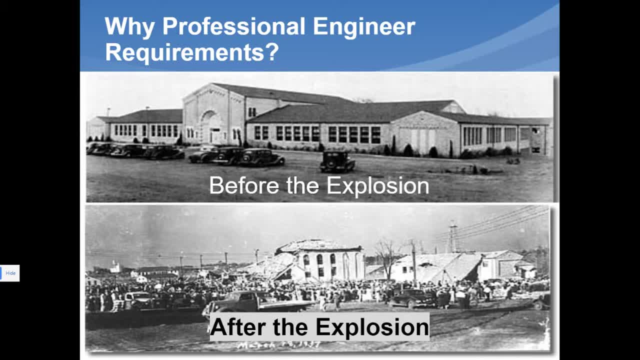 The explosion was heard for four miles away and out of 500 students and 40 teachers in the building, it killed 294.. Here on the slide you can see the before the explosion and then after the explosion pictures of the school. 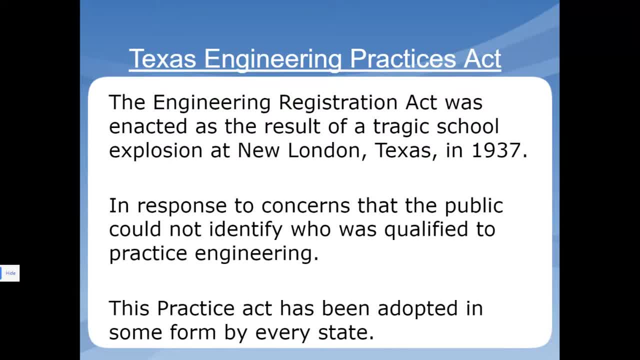 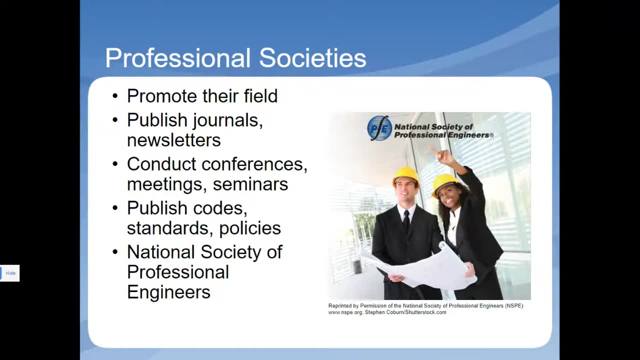 The Engineering Registration Act was enacted as a result of this tragic school explosion and in response to concerns that the public could not identify who is qualified to practice engineering. This practice act has been adopted in some form by every state, While the practice of engineering is regulated by states. 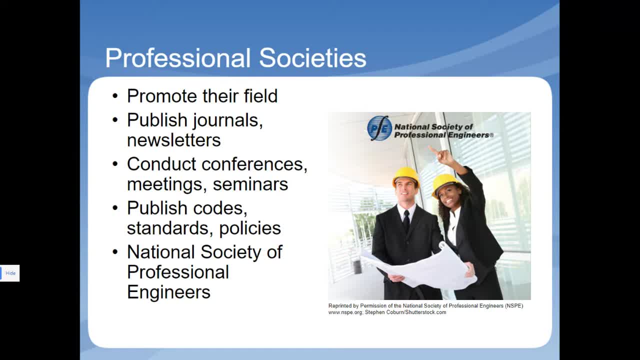 each field of engineering also has societies and associations. These organizations promote their field, publish journals and newsletters, conduct conferences, meetings and seminars, publish codes, standards and policies. Now, while most organizations focus on specific disciplines, the National Society of Professional Engineers. 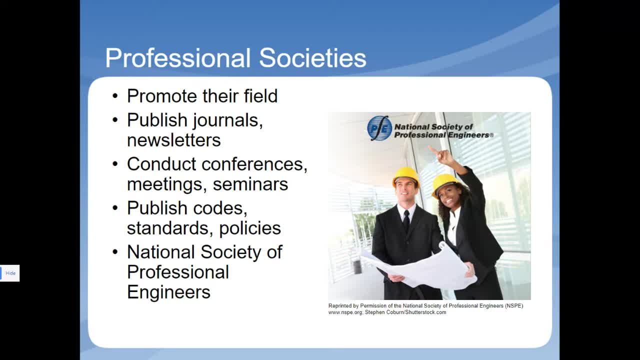 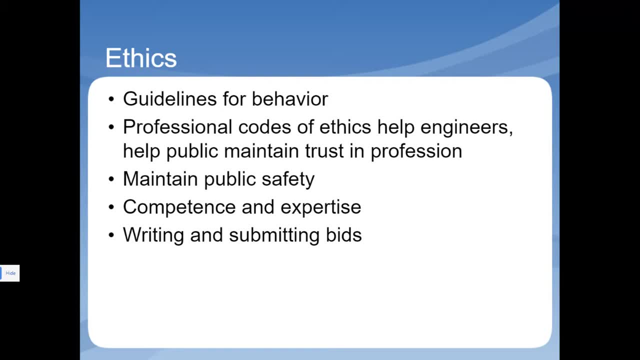 is a professional organization for engineers from any area of engineering. Professionals, such as engineers, face ethical decisions in their professional lives. Ethics are guidelines that we use to help make decisions about our behavior. In engineering, like most professions, codes of ethics are important because engineers have specialized knowledge. 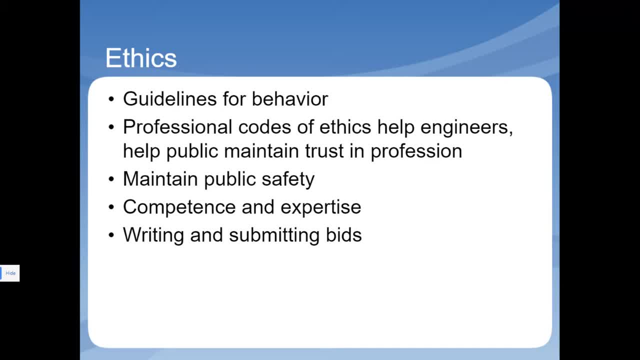 that the general public does not. Their knowledge, if used in unethical ways, could be harmful to the public. For example, it would be unethical or harmful for an engineer to create a new product knowing it is unsafe, while telling the public that it is safe.